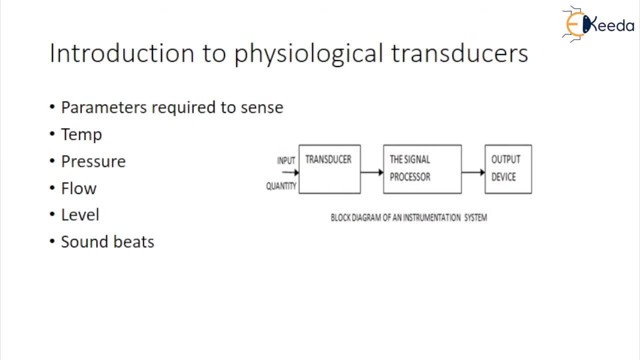 Transducer is a transducer which converts one form of energy into the another form. The basic parameters that can be sensed are listed. The first one is temperature, pressure, flow level and sound bits. The transducers are used to convert all these non-electric phenomena. 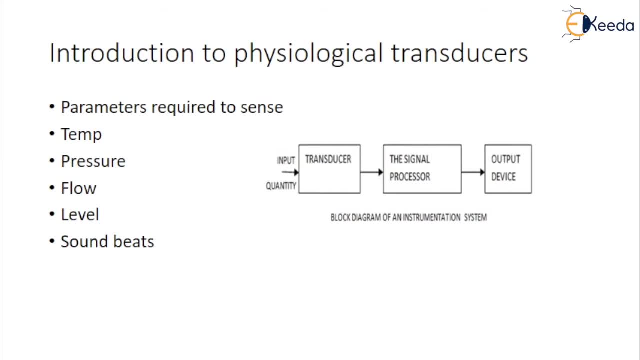 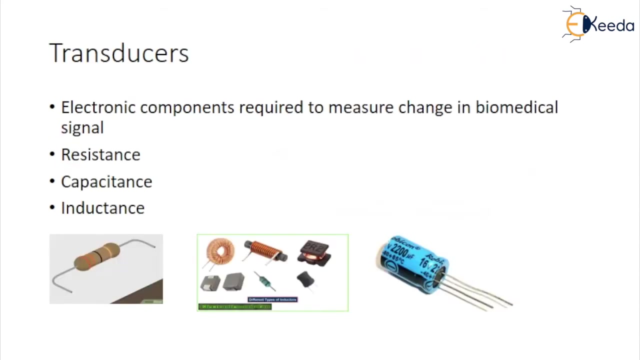 associated with the physiological events into electrical quantities. These biomedical signals from different parts of our body are further processed by signal processor and then transferred to the output peripherals such as visual monitoring, audio indication, Wi-Fi, Bluetooth, Internet connectivity for remote operations. The changes in the major biosignals can be detected by 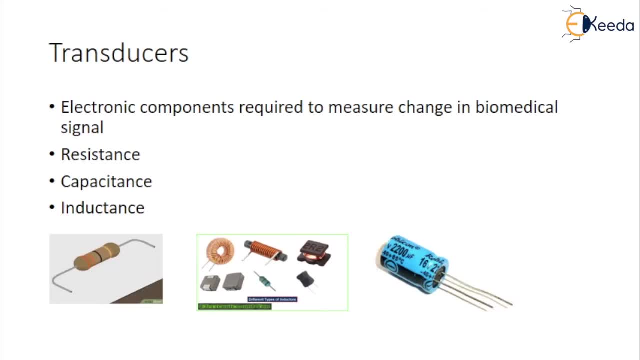 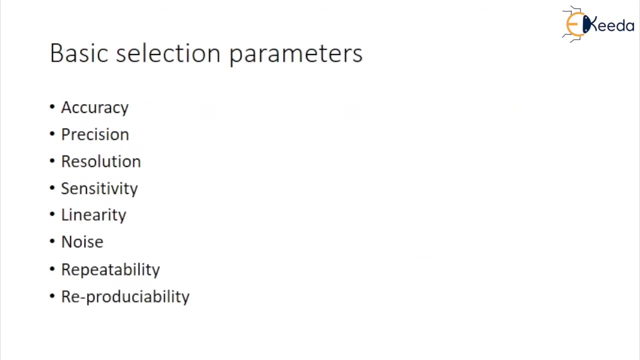 variation in electronic circuit parameters like resistance, capacitance and inductance. Piezoelectric and photoelectric transducers are commonly used for the measurement of biomedical signals. The basic parameters has to be considered while selecting proper transducers are listed below. These are: 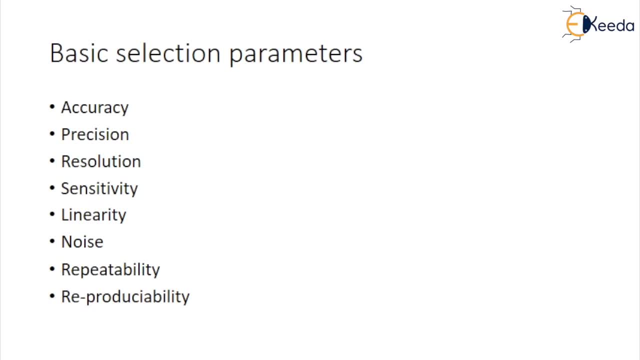 the static characteristics. The first one is the accuracy: It is expressed as a percentage of full-scale output. It is also defined as the algebraic difference between the reference value and the measured value. Second is the precision: It gives degree of repeatability of measurement. Resolution: It indicates the 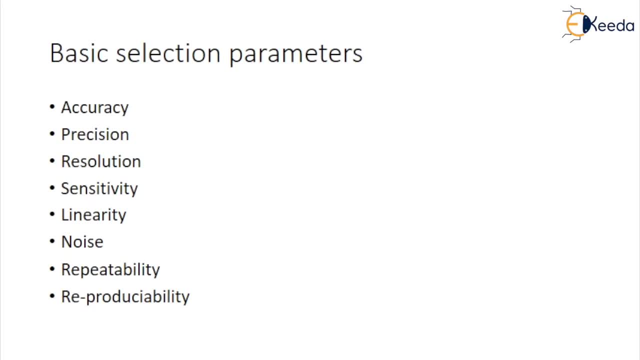 smallest measurable input Increment Sensitivity Describes transfer ratio of output to input Linearity. It reflects the output proportional to the input Noise. This is an unwanted signal at the output due to either to internal source or to interference Repeatability. It is the result of success. 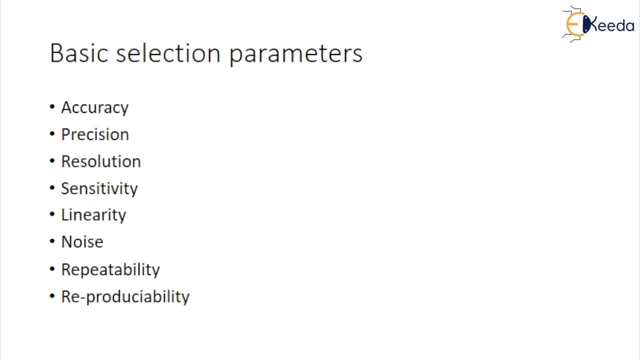 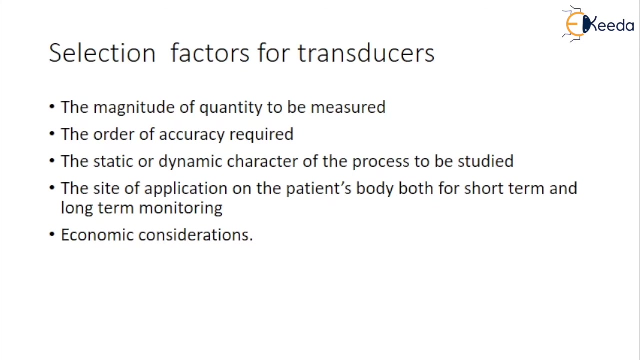 you: measurement of same variable carried under same measurement conditions. Reproducibility: It is the result of successive measurement of same variable carried under different measurement conditions. Now let us learn the factors on which the selection of transducer depends for the study of a specific 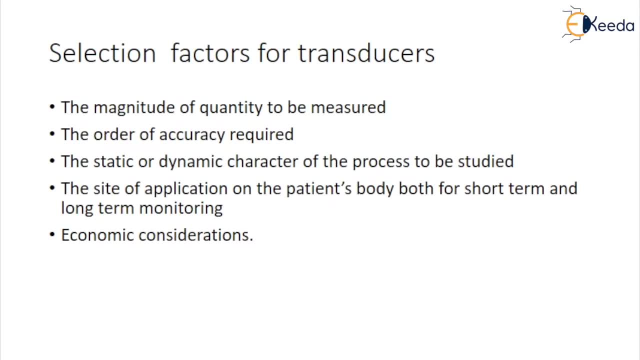 phenomena. The first one, the magnitude of quantity to be measured. Next the order of accuracy required Means- in such a difficult conditions, students, the very important parameter has to be measured is the variation in body temperature. So selection of temperature sensor is such that it measures body temperature with 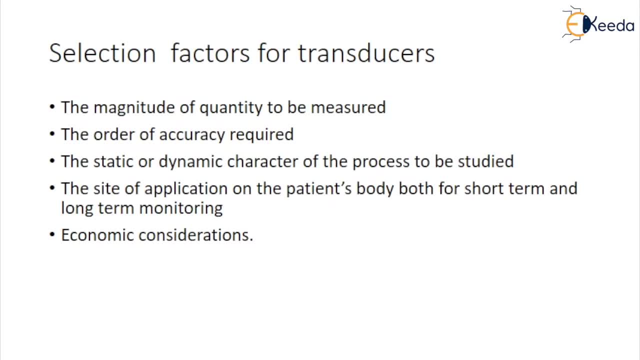 very high accuracy. Next, the static or dynamic character of the process to be studied. The selection of transducer depends on the process parameters, which does not change with the time or change with respect to time. The site of application on the patient's body, both for short-term and long-term monitoring means. 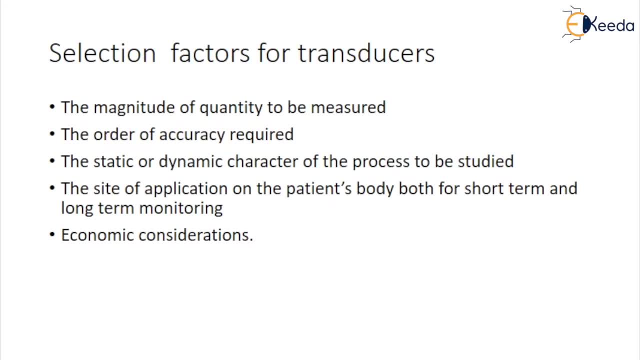 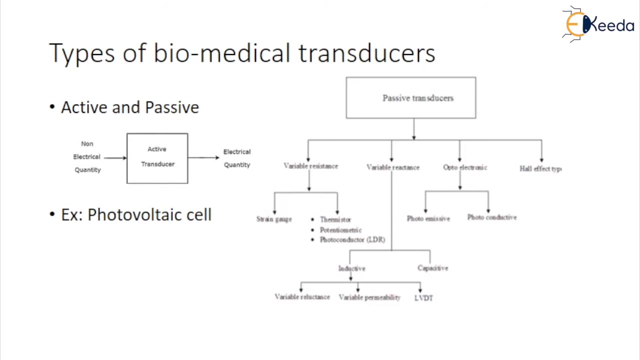 effect of application of such transducers on the patient body for short and long term period. The last and the most important factor is the economic consideration. Such transducers must be economical and easily available in the market. In the medical field, many physical, chemical and optical properties are used to construct biomedical transducers. 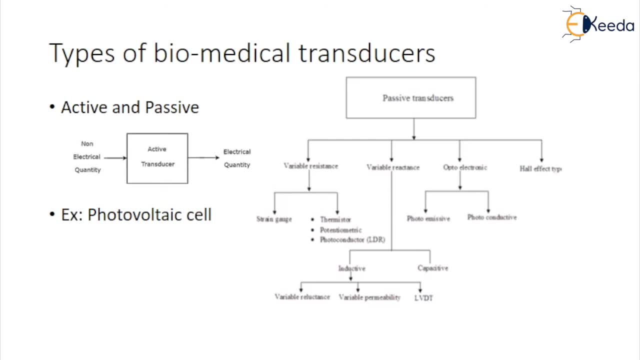 Basically these are divided into two major categories. The first one is active transducers and passive transducers. The active transducers are those which directly convert non-electric quantity into electrical signal. They do not require an external electric supply for the conversion. For example, photovoltaic cell. Photo means light and voltaic means electric. 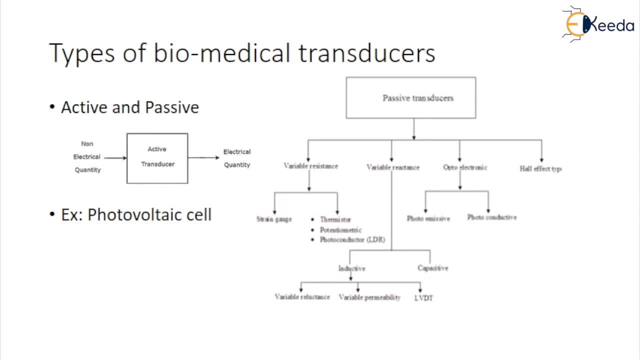 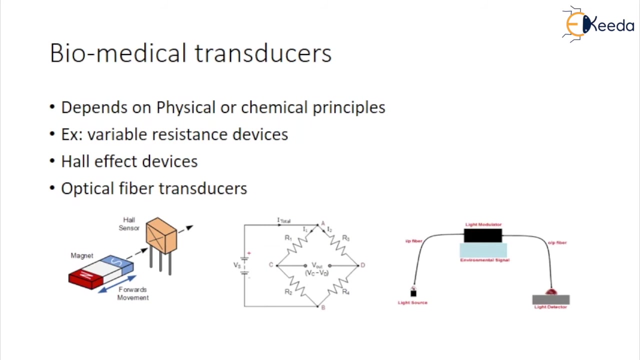 energy. so light energy is converted into electrical energy in passive transducer required an external electric supply for conversion process. for example, variable resistance connected in whittstone bridge which requires an external ac or dc supply to operate. have you understand the concept of active and passive? okay, then we'll switch again. it is subdivided, depends on physical. 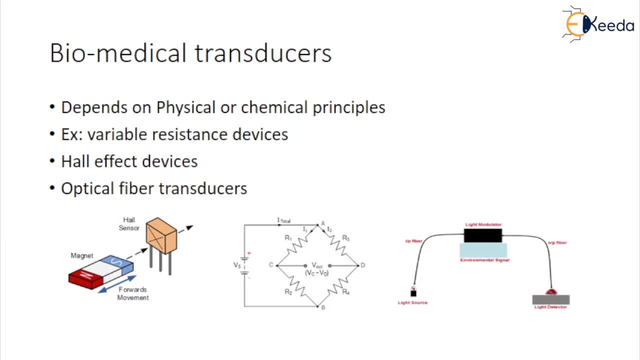 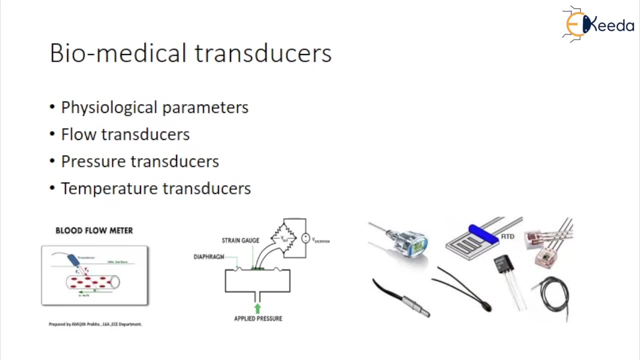 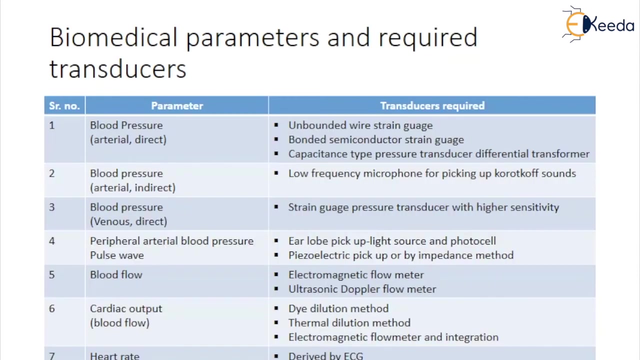 or chemical principles, for example variable resistance devices, hall effect devices and optical fiber transducers. for measuring some physiological parameters, we are using flow transducers, pressure transducers and templates temperature transducers. Let us learn an interesting part from biomedical parameters and the transducers which are used for their measurement. The first one is blood pressure. 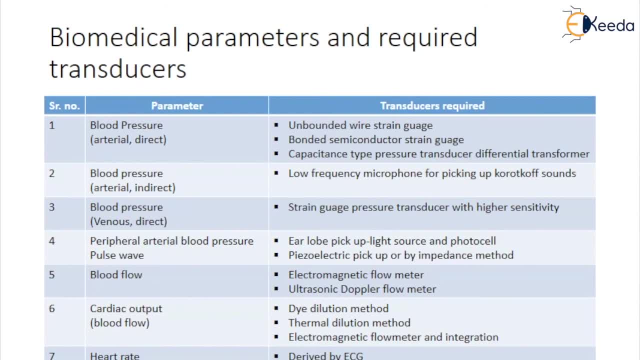 measurement, that is, atrial blood pressure and direct measurement, and the transducer is used is unbounded via strain gauge or we can use bounded semiconductor strain gauge or capacitance type pressure transducer. differential transformer. Second one is the same blood pressure measurement, but it is an indirect type of and the transducer used is a low frequency microphone for picking up. 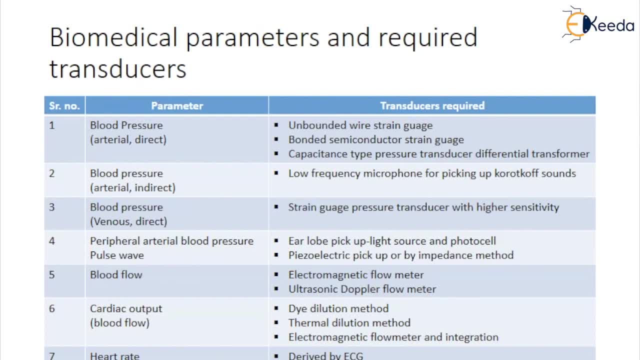 Korotkov sounds. These Korotkov sounds are nothing but the lub dub sounds created by the opening and closing of heart valves. Next is important blood pressure venous distribution. This is the blood pressure venous distribution. This is the blood pressure venous. 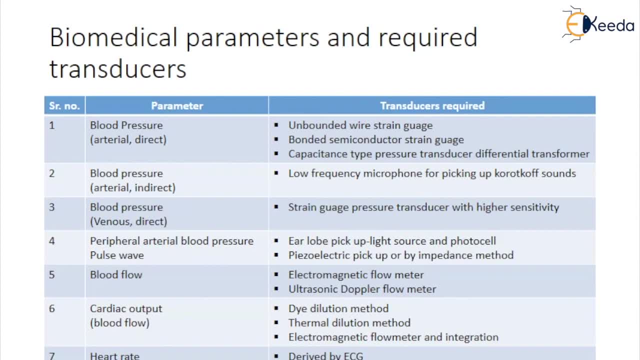 direct, And for these we are using strain gauge pressure transducer with very high sensitivity. Next is peripheral atrial blood pressure pulse wave, And for these measurements we are using a light source and photocell and piezoelectric pickup. Very important parameter is the blood flow.